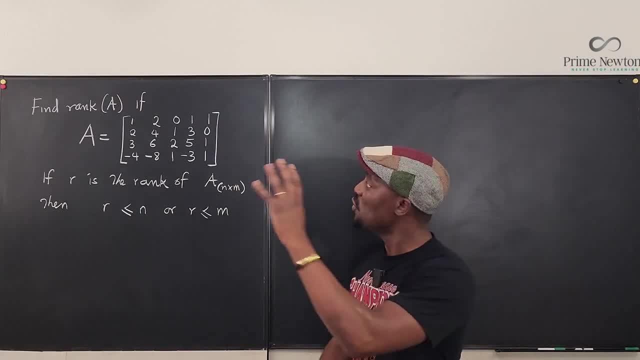 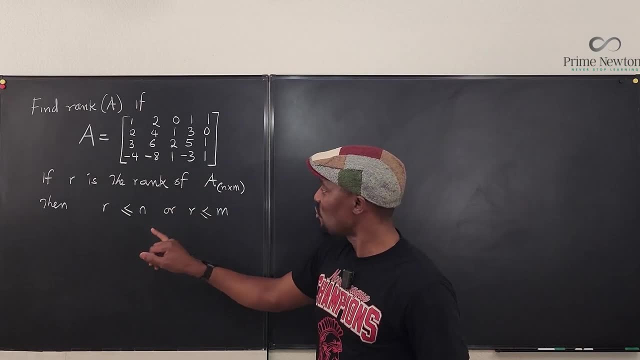 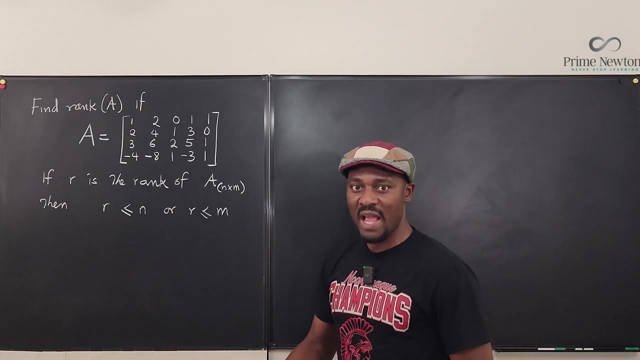 So it is. whichever is smaller, that R will be. So you, looking at this matrix, automatically tells you that the rank of this matrix has to be four or less, because this is a four by five matrix. Now, what really is the rank of a matrix? It's a four by five matrix. It's a four by five matrix. 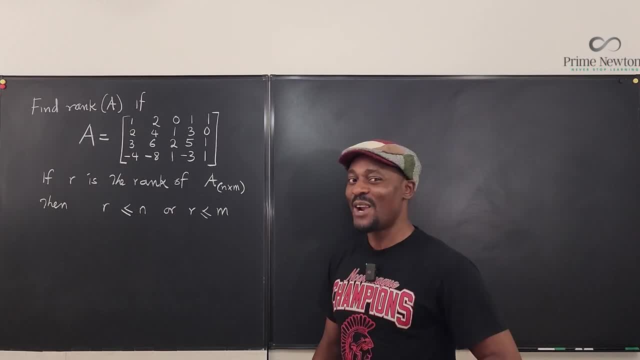 How do you get the rank? Or how do you get the rank? Okay, I don't want to go into all the definitions, but there's this corollary of a theorem. I'm not going to talk about the theorem. I just want you to know that any matrix you see ever, you can transform that matrix into the. 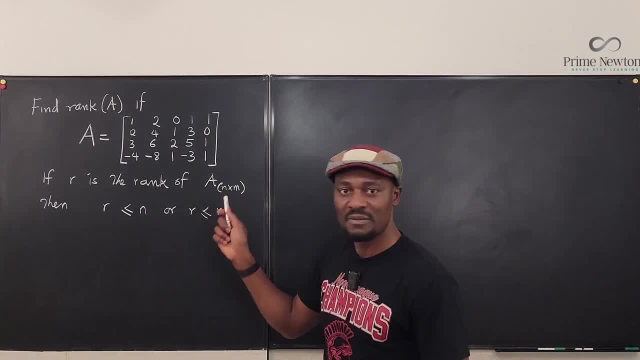 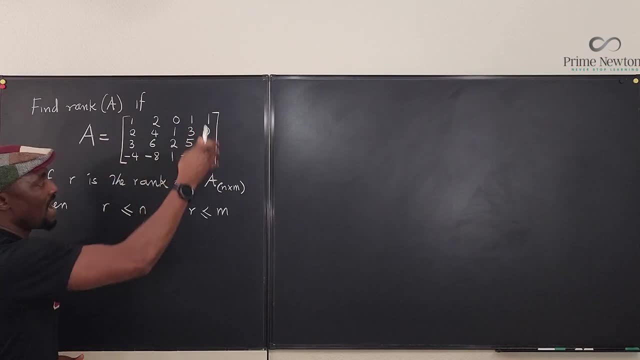 identity matrix of the smaller dimension. So see what this means, because this is a four by five matrix. It's a four by five matrix. It's a four by five matrix, It's a four by five matrix. What we're saying is that you can actually transform this matrix so that it becomes, at most. 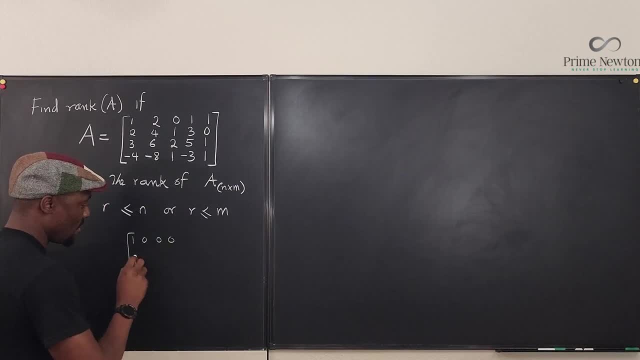 it's going to be 1, 0, 0, 0, 0, 1, 0, 0, 0, 0, 1, 0, 0, 0, 0, 1.. And then you're going to have zeros. 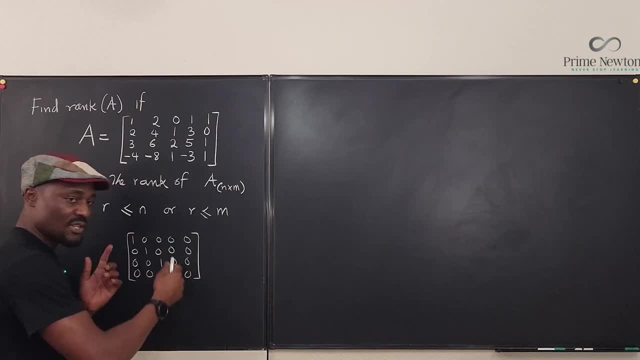 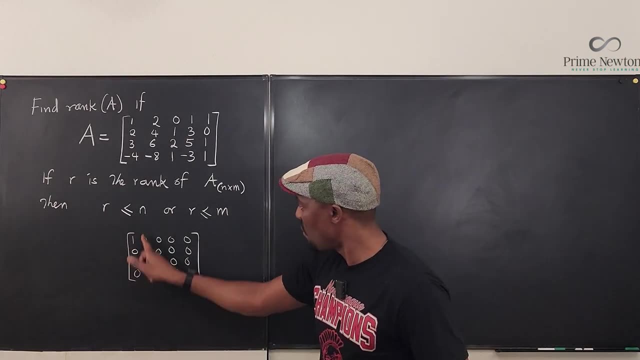 here, because this is a four by five matrix. This is the best you can get, And if you get this, it means the rank is four because the rank is four. So if you get this, you're going to have there are four linearly independent columns or four linearly independent rows. 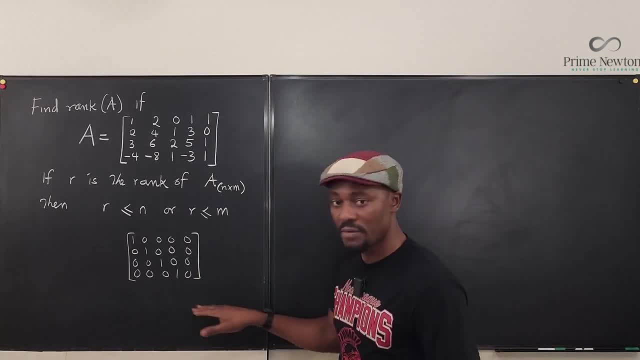 You're going to have a column of zeros or a row of zeros, depending on which one has more, because you have five columns and four rows, definitely there'll be a column of zeros. But if it was flipped, if it was N by N, then you're going to have a row of zeros. 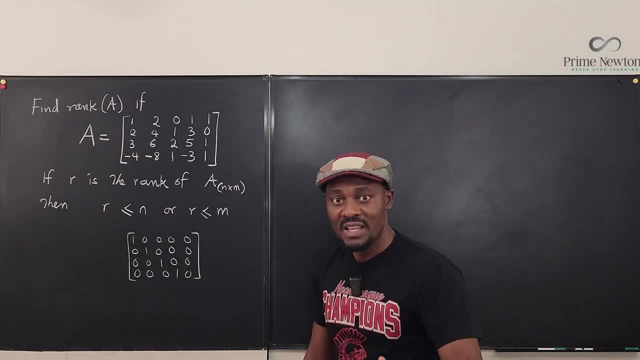 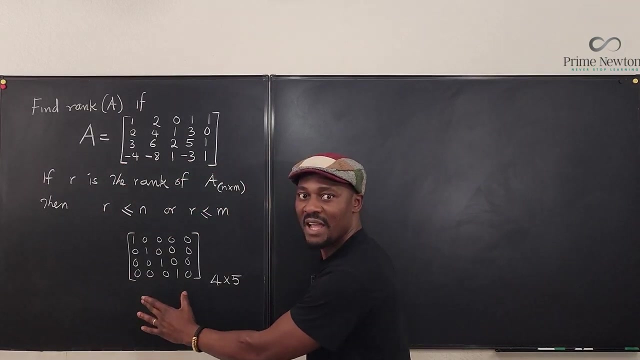 So, basically, this is what the theorem says, But this is the best you can get. Remember, the rank is less than or equal to N. In this case, our N is four. This is a four by five matrix. So this is the most you can get. It is the four. 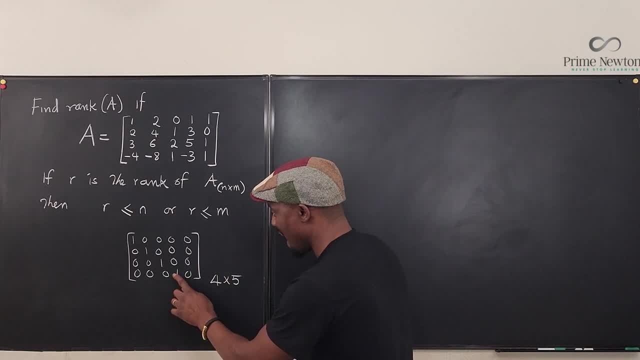 It's possible that it is less than four, such that even this one is going to be a zero, So that you're now going to have one row of zeros and two columns of zeros, so that the most you get will be just three linearly independent rows, or three linearly independent columns, or three pivots. 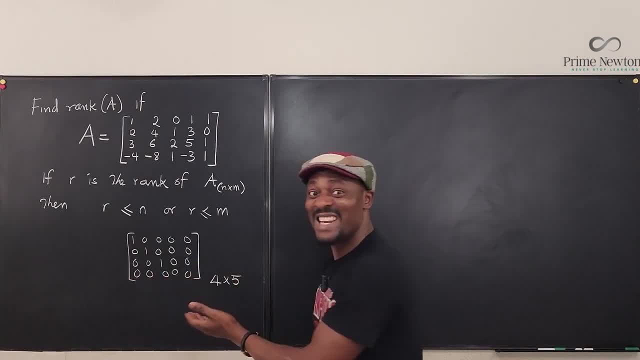 Remember we talked about pivots the other day, and that's it. They all have equivalent implications. It's even possible that this also is zero, So that you only have two linearly independent columns. It's even possible that this is zero. 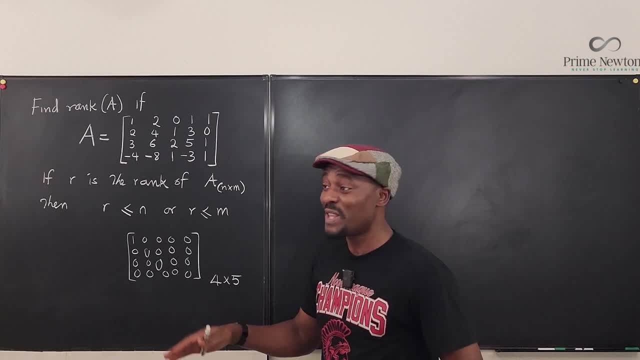 So that all you have is just one column or one row that was duplicated three times, and then you had four by four rows. I mean you have four by five, or it could be just be one column that was duplicated four times and then you had five columns. 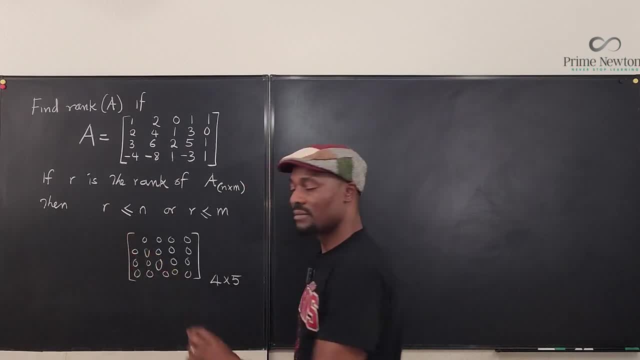 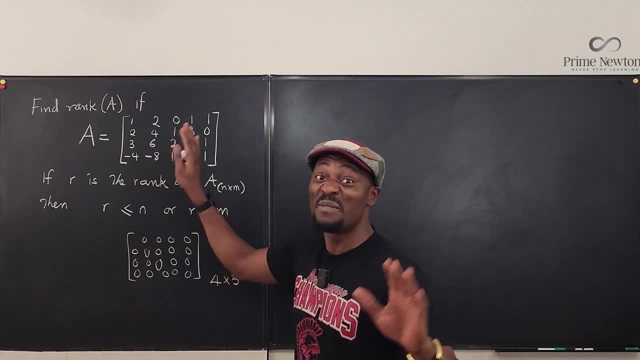 Now, is it possible for this also to be zero? This is never possible unless everything here was a zero in the first place. Yes, if all you had was zeros, then this is what you. you don't need to do any work. 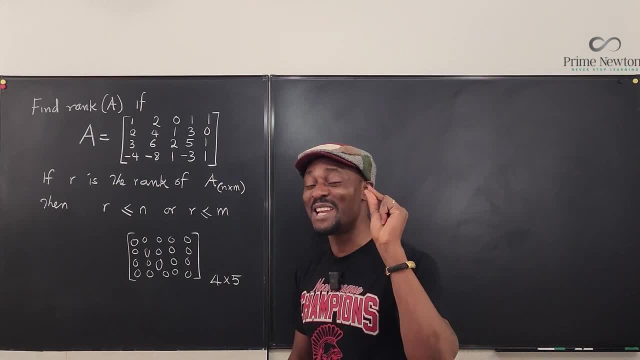 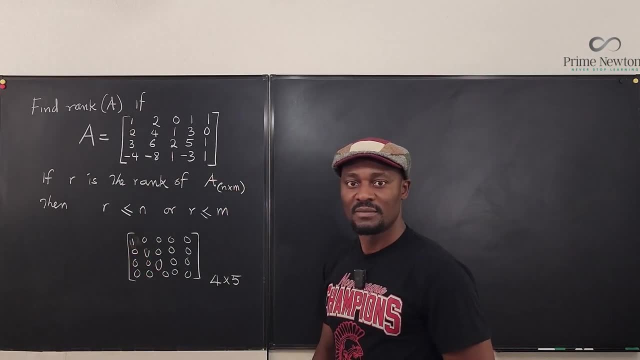 But as long as one non-zero entry was made in a matrix, you definitely can have all zeros. There has to be just some one somewhere, a minimum of one. Now let's say this is all you got, after you simplified. Then you say: because there's only one row. 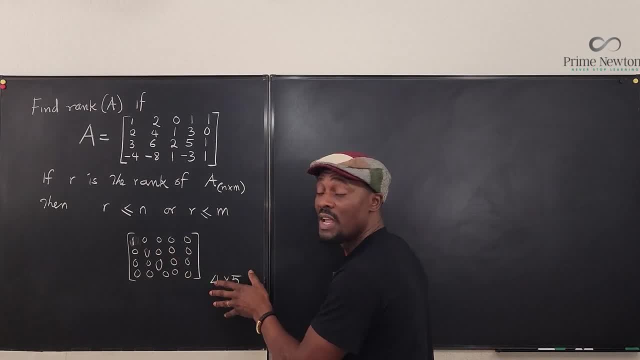 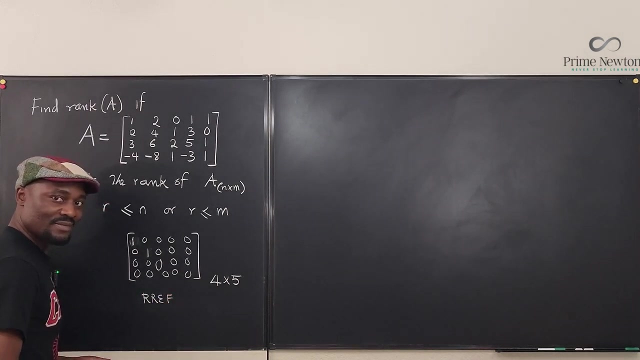 that has a pivot, everything else is zero, then the rank of this matrix is one. If you are able to generate another one here, remember this form we're talking about is the reduced row echelon form. Okay, so that's why we learned it in the previous video. So if you're able to write this as 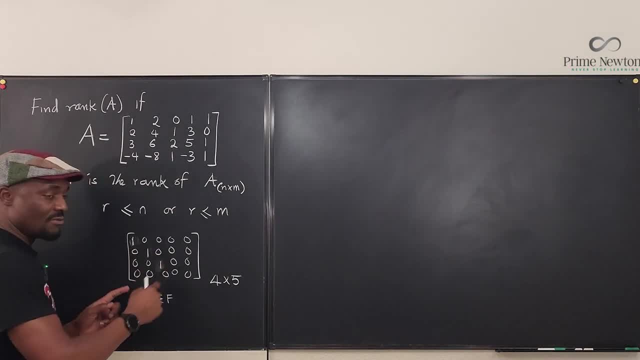 then you say that this has a rank of three. If you're able to generate this last one here, then it has a rank of four. But don't forget that you would always go by the smaller number. Now, if it's a square matrix, a three by three, 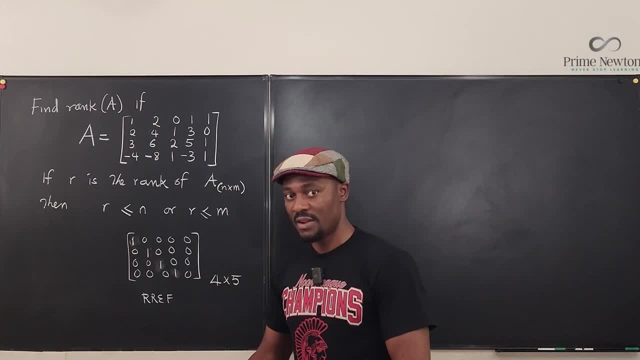 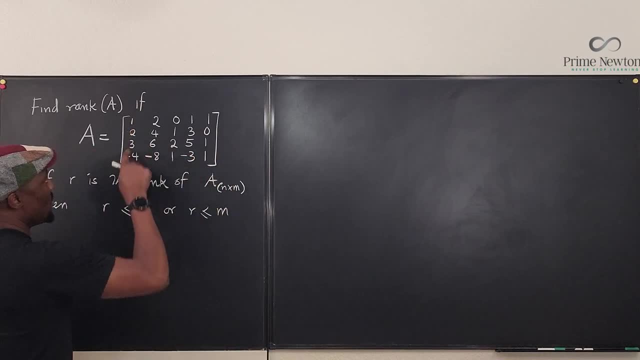 then you expect to get a four, a three or two or a one. okay, that would be the rank of the matrix. so let's do the work on this one. now. what we do is we need to create zeros here, okay, so i'm going to. i'm going to do two. 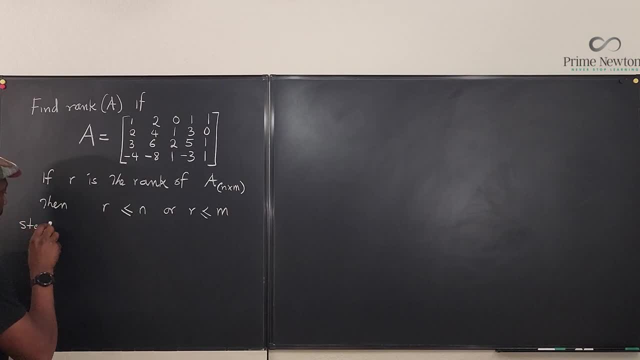 on this side. so let's go steps. we're going to say so. the first matrix is going to have one two, zero one one. we need that, okay. so what do we do to this one? we're going to add minus two of this to this. so let's say plus. let's say minus two. minus two r one. let's do it that way. so minus two. 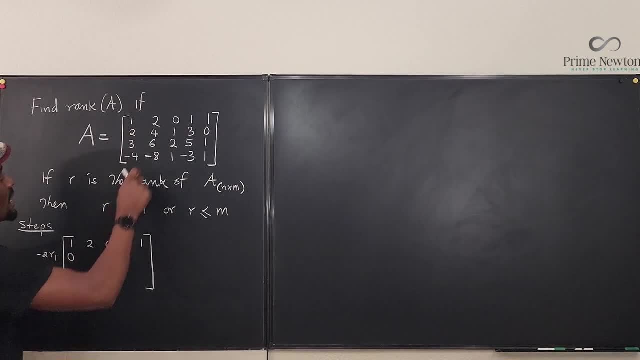 r one is going to be: this minus this gives you zero. this minus two of this gives you zero. this minus two of this gives you one. this minus two of this gives you one. this minus two of this gives you minus two. nice, the next one. oh, it's gonna be minus three r one, so there's gonna be. 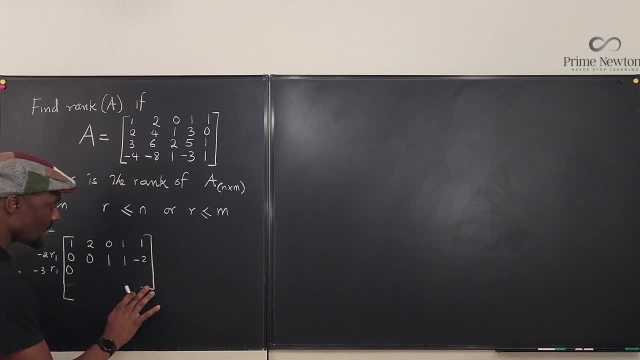 zero. i'm gonna extend this a little. okay, we're gonna have zero. six minus three of this is gonna be zero. uh oh, it's beginning to look familiar. this minus three of this is two. um, this minus three of this is two, and this minus three of this is minus two. okay, one more. what do we do? 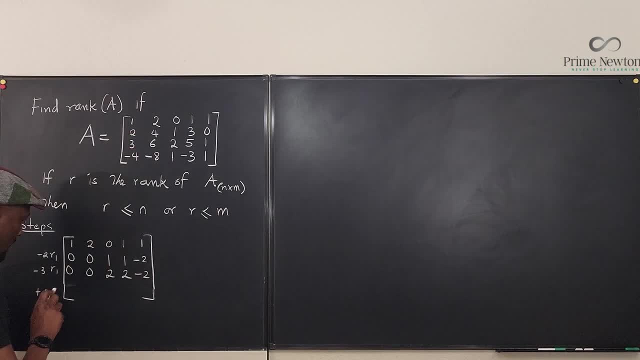 we're gonna add four of this to this, so plus four r one. so if we add four r one to this, what do we get? we're gonna have zero. um. this plus four of this is zero. this plus four of this is one. um. this plus four of this is one. and finally, this plus four of this. 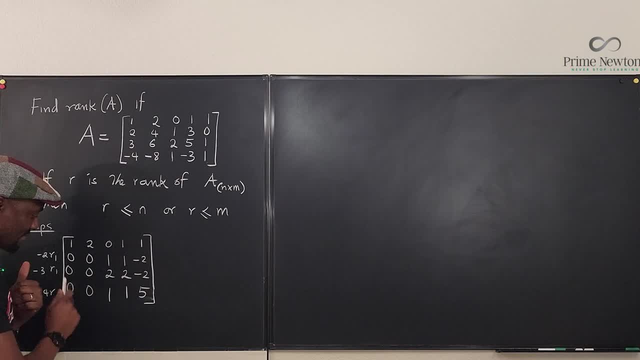 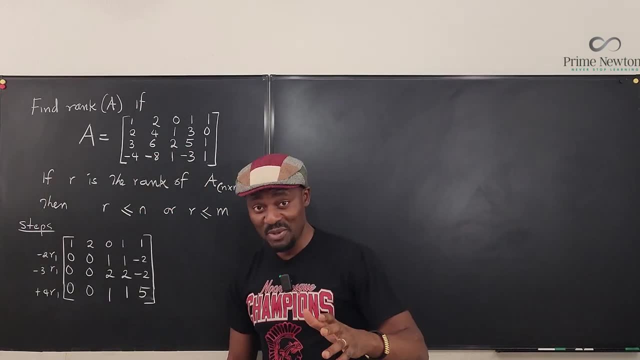 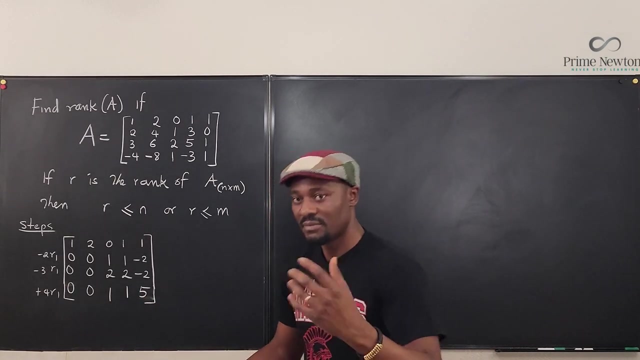 is five. nice, we already have this automatically done for us, so we need another. oh, the pivot. remember, remember this, that in row echelon form, let's just go straight to reduce row epsilon form, row echelon form. we're gonna have this. this is not a pivot. so we look for the next number in. 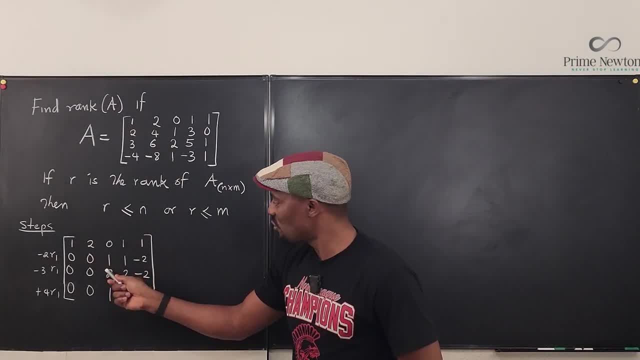 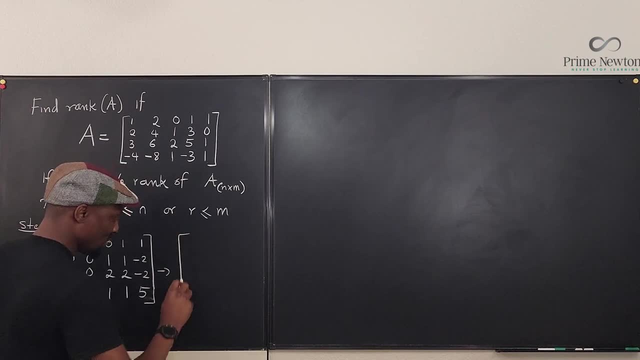 the next row. this is the first number, so we have to make anything under this a zero. so what we're gonna do next is this: let's see if i can squeeze that in here. so, um, what we're gonna do because? so we're gonna leave the top. let's leave the top alone. 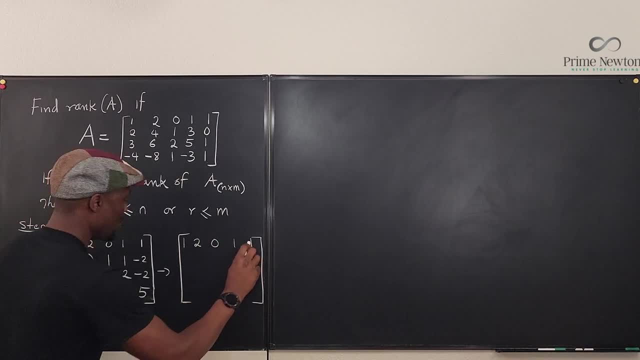 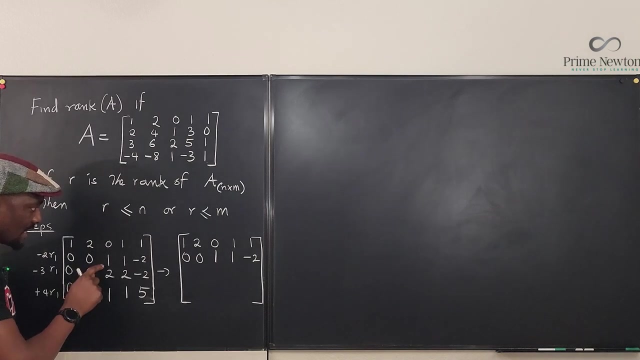 one, two zero one one. we're gonna leave the next row zero, zero one. one minus two, the middle row. we're going to eliminate this here and put zero, make a zero here. so we're going to add: let's say here what do we do? let's put it here because i want to write what i'm doing next. so 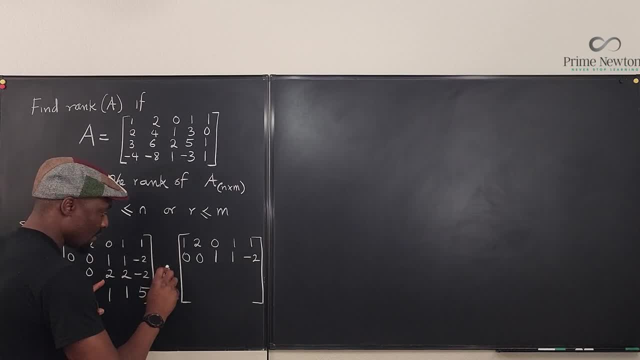 here i'm going to add minus 2 r1 to this. minus 2 r1. i don't like my notation, but just understand that that's what i did to get this. so this, not r1 minus 2 r2, because it's this one, so i have this. 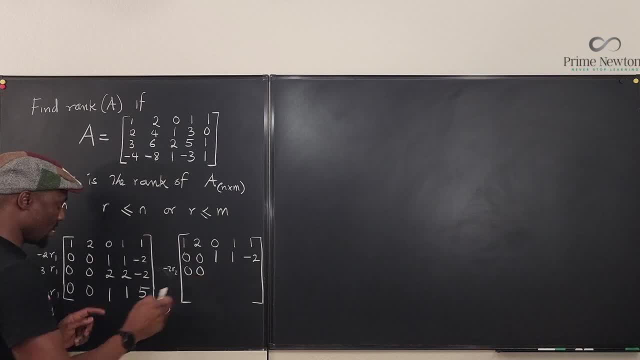 zero here and i have the zero here, but at this point i have minus two. this minus two of this gives me zero, this minus two of this gives me zero, and this minus two of this will give me two, nice, and then i go to the last line. i have zero, zero. now what i need is add minus of this. 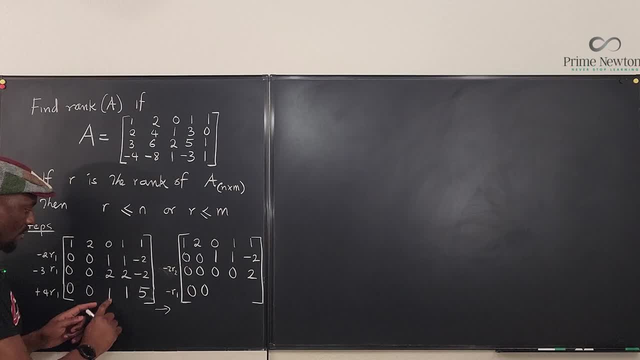 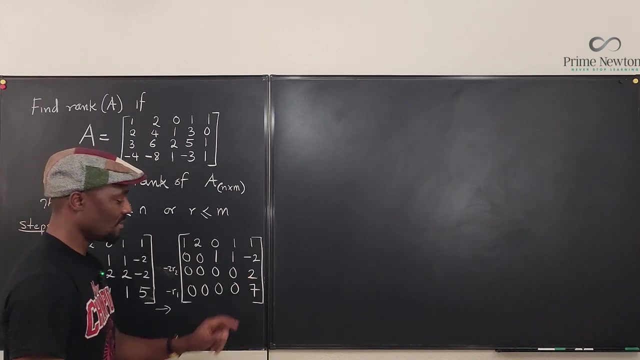 to this. so minus r1. so if i do one minus this gives me zero, this minus this gives me zero, and five minus this gives me seven. okay, so now i have a pivot here. i have a pivot here. well, no, this is the next one that's gonna be a pivot for me. so what i'm going to do is this is a two. so you see. 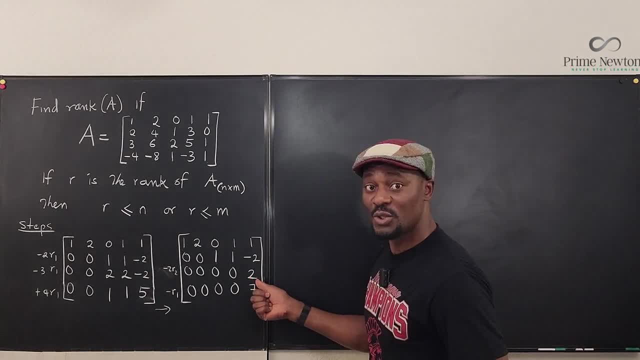 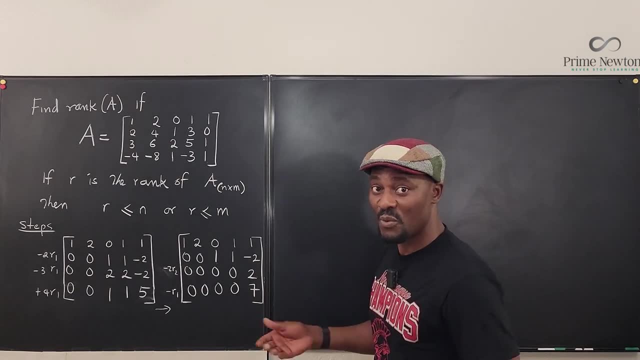 where it's not easy to work with two. so what i'm going to do is divide this by two, so that what i get will be one and i can use the one to eliminate the other one. so i'm going to divide this by two now, because i'm doing reduced row echelon form. i think i should have gotten rid. 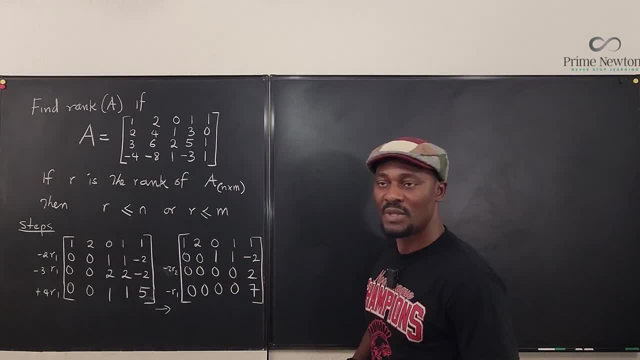 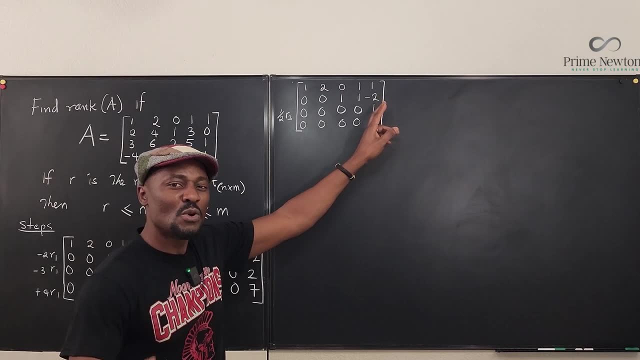 of well, nothing. let's make this a one, okay. so we're gonna say okay. so what do we do next? i need to get rid of- because i'm doing reduced row echelon form at this point- i'm just gonna get rid of everything that's in front of it. let's go back to the traditional notation. 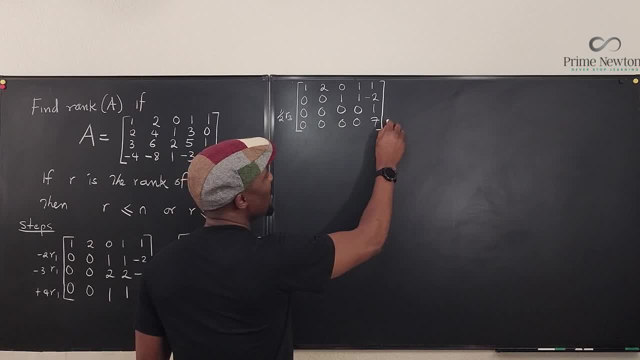 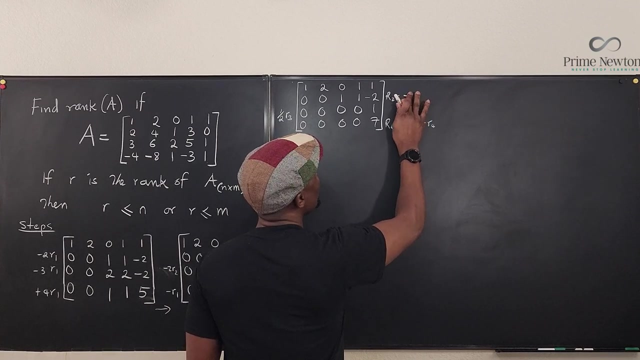 okay, so i'm gonna say that this new row, row four, is equal to minus seven. row three plus row four, and i'm gonna say this is gonna stay, i'm gonna get rid of this. that's gonna be um. row two will be equal to minus will be two. row two will be two. row three: 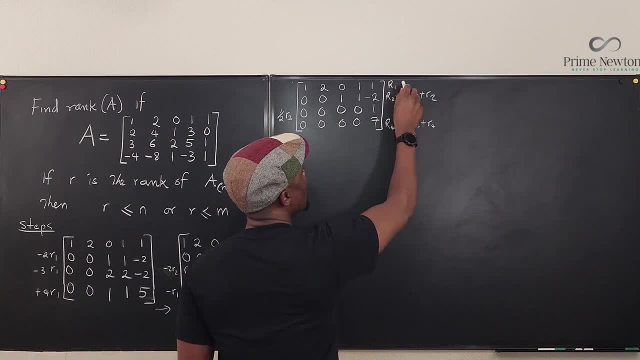 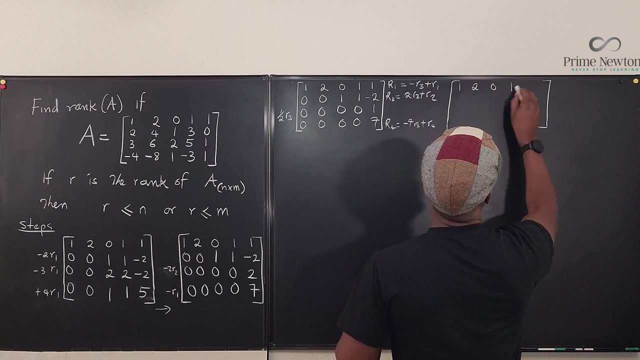 plus row two, and this is going to be row one, and it's going to be equal to minus row one plus row three plus row three plus row one. okay, so let's write out what we get. we got one two zero, one zero. the next one is this: we're going to get rid of this. 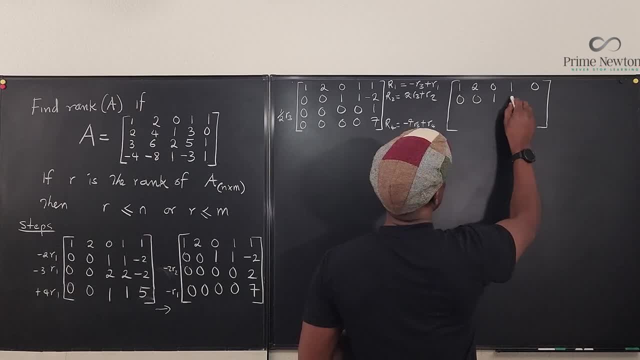 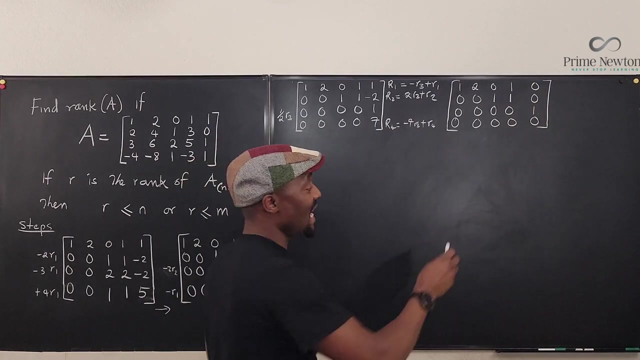 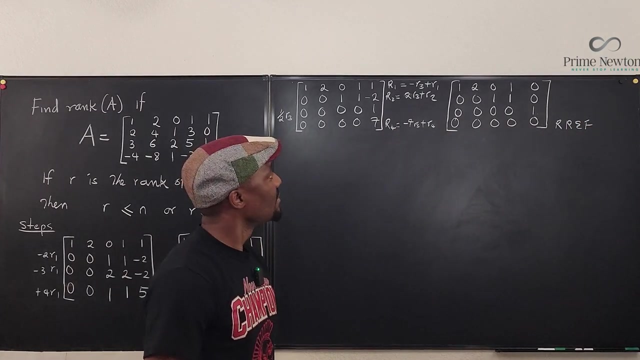 it's going to be zero, zero, one, one, zero. and then we go here, we're gonna get zero, zero, zero, one, and finally we're gonna get zero, zero, zero, zero, zero. this is not a pivot, this one. we've gotten rid of everything. so this is in reduced row echelon form. we don't need to worry about this. 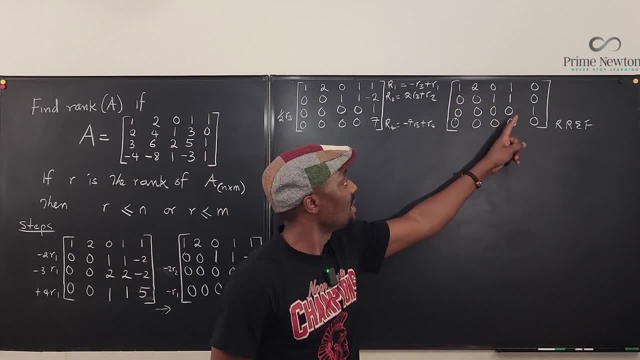 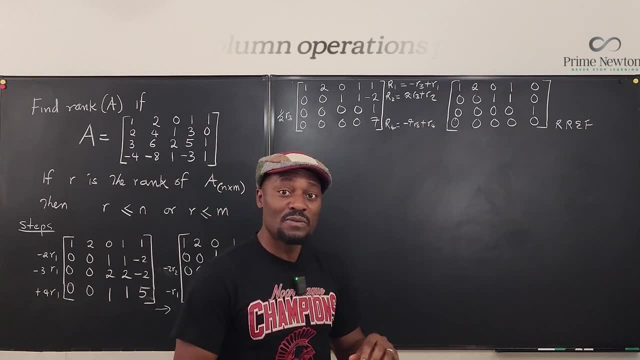 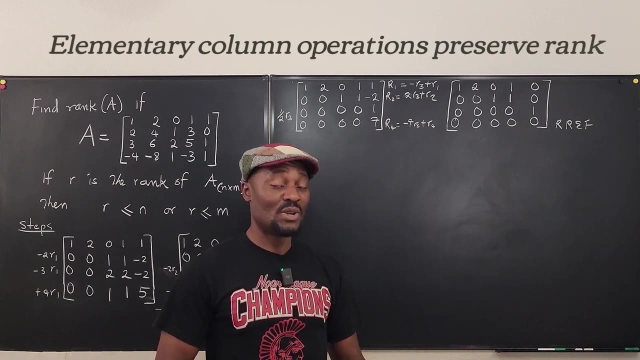 because it's not a pivot. so this is a pivot, this is a pivot. this is a pivot. there are three pivots. take this and once we remove this pivots, we will see two. my leaning, it's a pivot, it's a pivot, it's a pivotsع y nos per zero. zero one two is equal to six above zero. 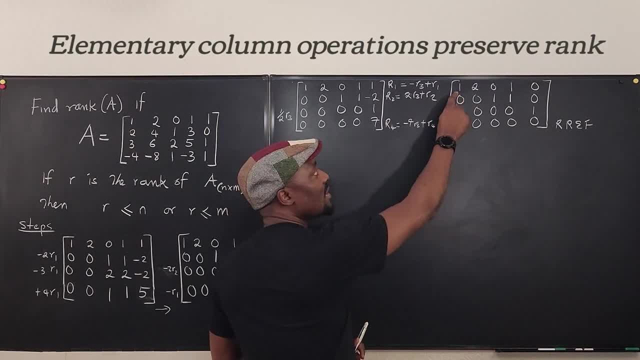 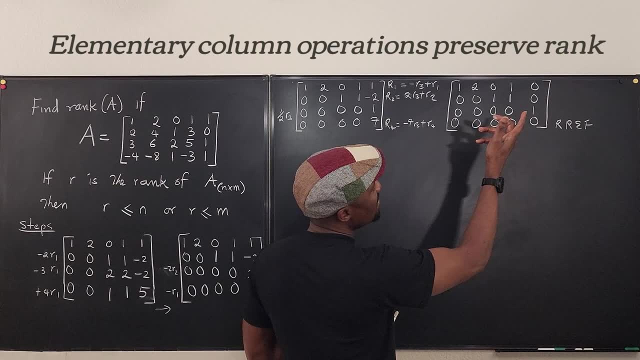 this is not a pivot, this is not a pivot. right two is equal to six, and so we've taken the still from the initial order. four: choose some columns, go and take them. you have five columns in your pattern and you have three columns. so this is a pivots and this is not a pivot. and that marry to. 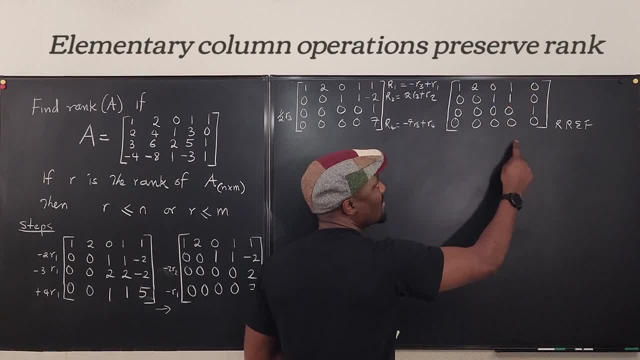 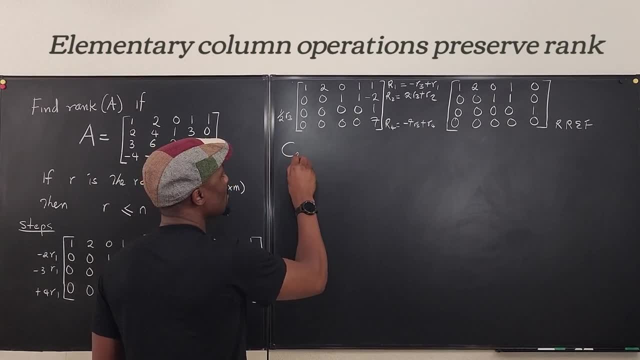 I can get rid of this column and this column And watch what I'm going to do. I'm just going to write it here. So I'm going to say the new column 2, this column can be the same thing as minus 2 of the old column, 1 plus the old column 2.. 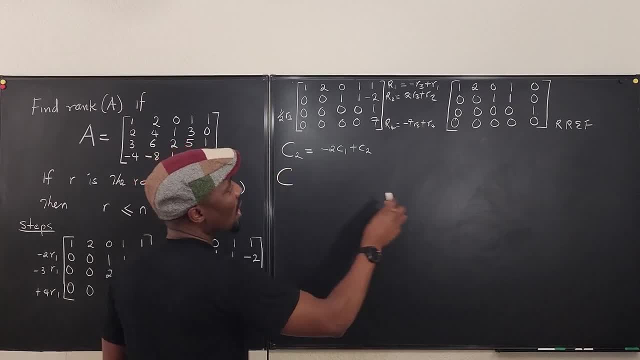 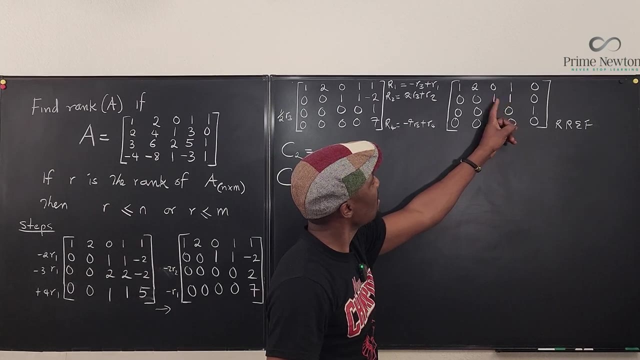 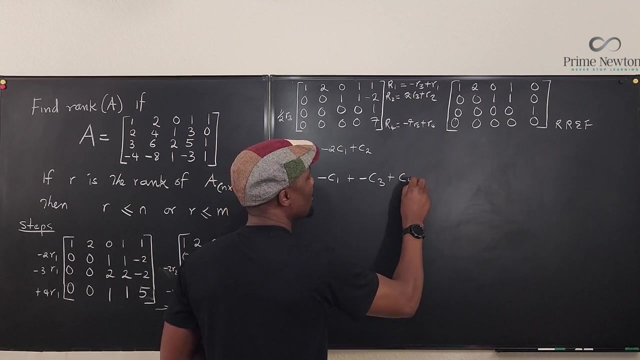 And I can also say that the new column 4 can be written as: ah, watch this. minus column 1 plus minus. let's see. we want to get rid of this minus column 1 plus minus column 3 plus the old column 4.. 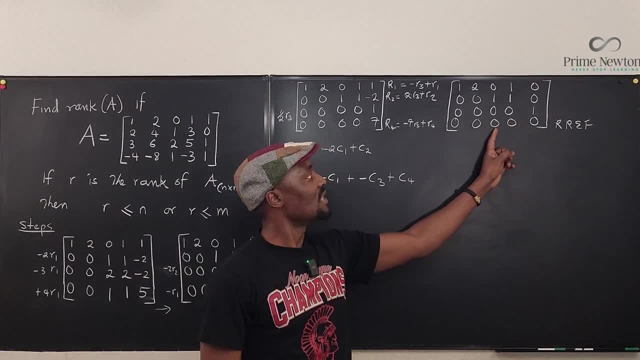 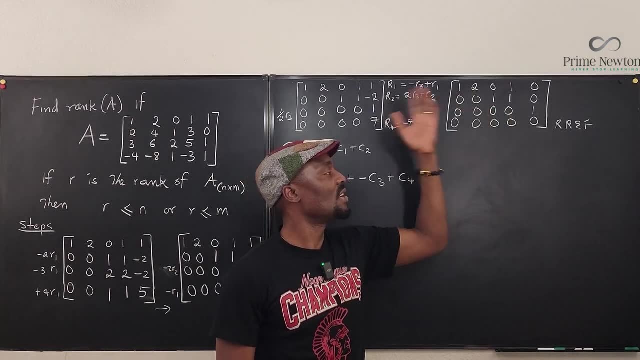 So I can get rid of this by subtracting this and subtracting Subtracting this from it. it's going to go to 0.. I can get rid of this by subtracting 2 of this from it. It's going to get to 0.. 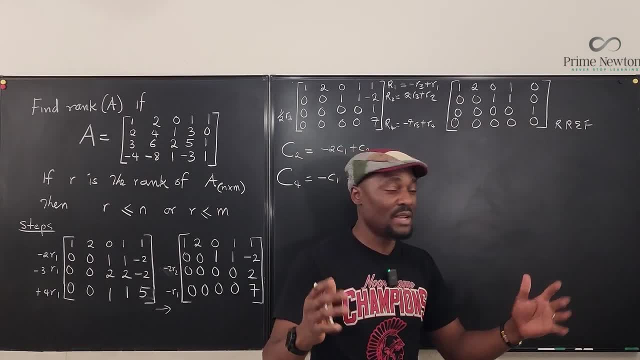 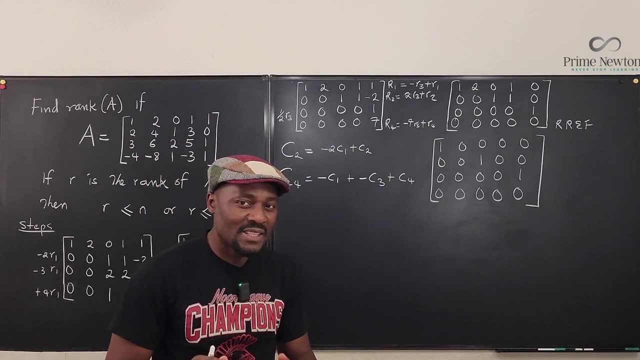 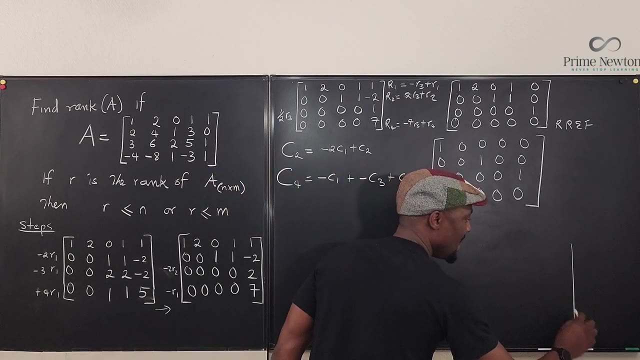 There's no other column you can subtract And then you're going to see a good picture that we have. See what we have. It's going to become 0. And that's what you are left with Now. remember what I said: that you can push everything to one corner so that at the end of the day, you're going to get a matrix that has four sides. 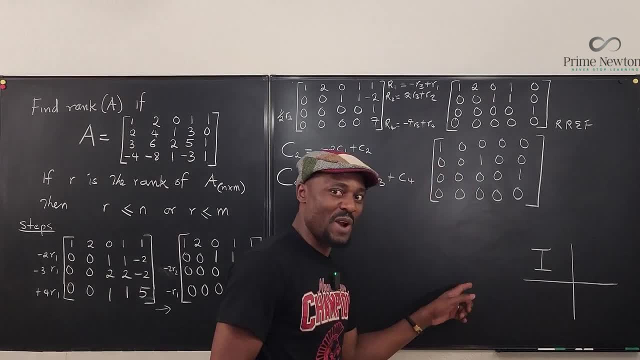 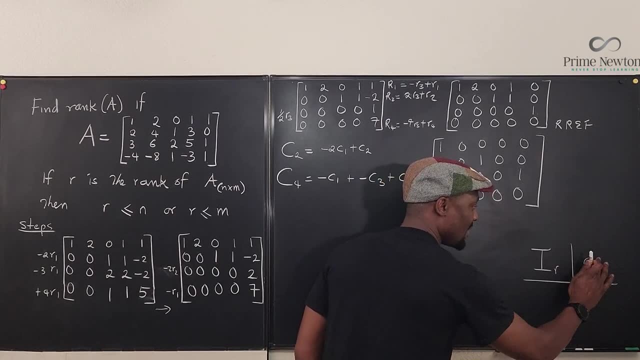 One side is the identity matrix for the column Or the rank that you're looking for, and then you're going to have some zero matrices here. Let's call this I I don't want to use I. let's just call it N1,, call this N2,, call this N3. 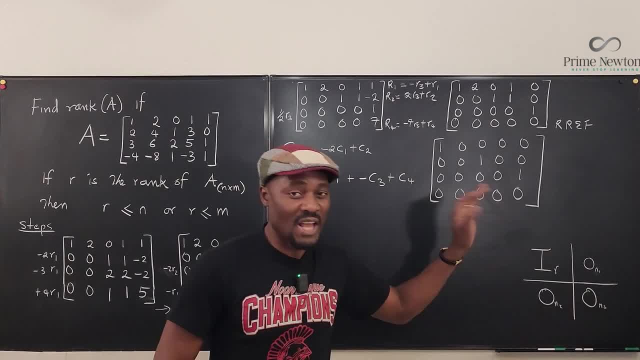 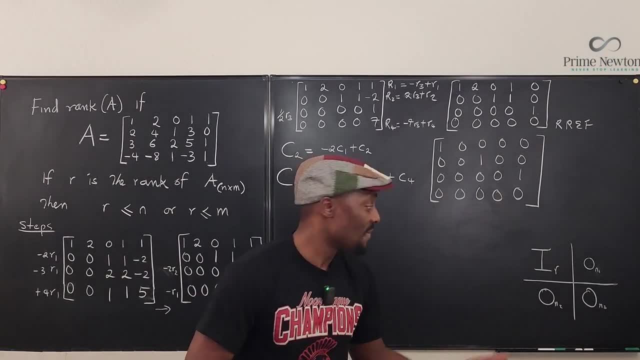 This is just the number of rows and columns they have, or their dimensions. I don't know what they are, but this is what you're looking for. Whatever this identity element has as its dimension, dimension is the rank of the matrix. So look at this. 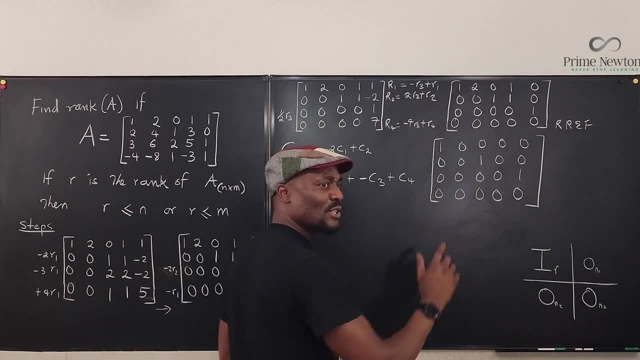 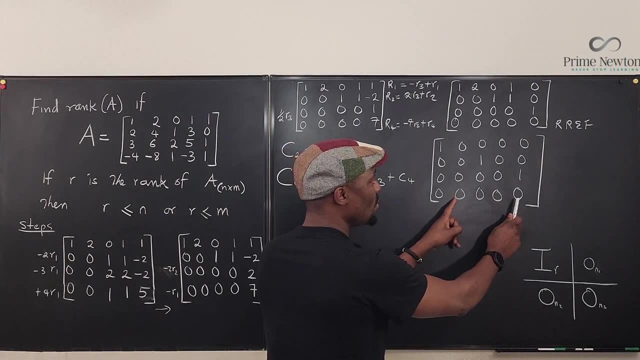 How can we get? we don't need the zero here. So we can do elementary column operation, which is just switching rows. So we can switch row two and row five. No, we can switch row two and row three and then bring this guy here. 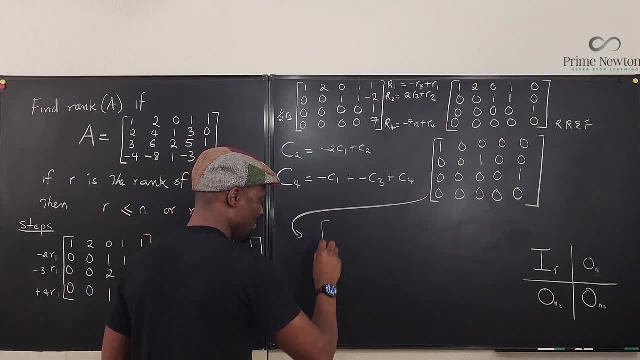 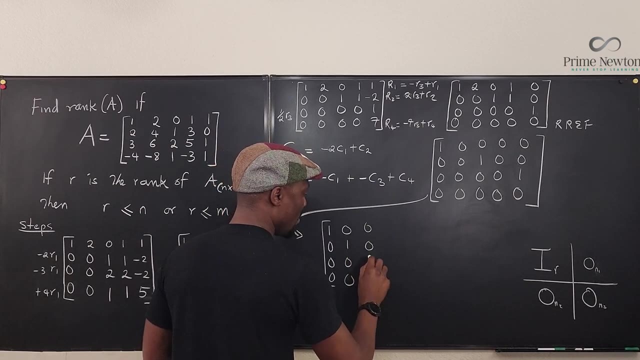 So this can actually be written as 1, 0, 0, 0.. 0, 1, 0, 0.. So I'm bringing this here and then I'm going to move this here, or 0, 0, 1, 0. 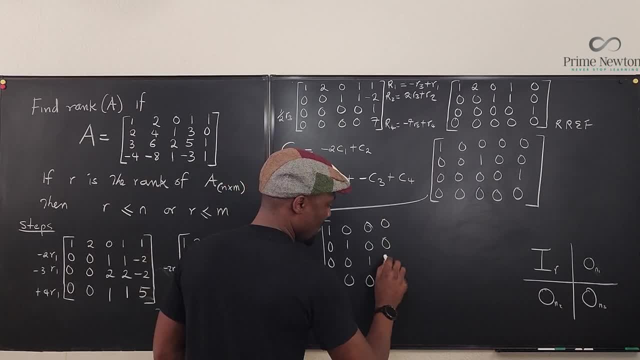 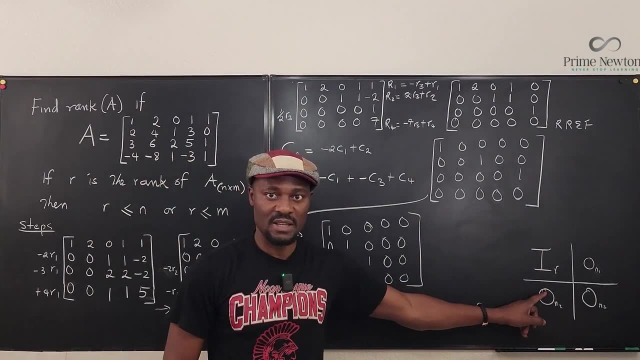 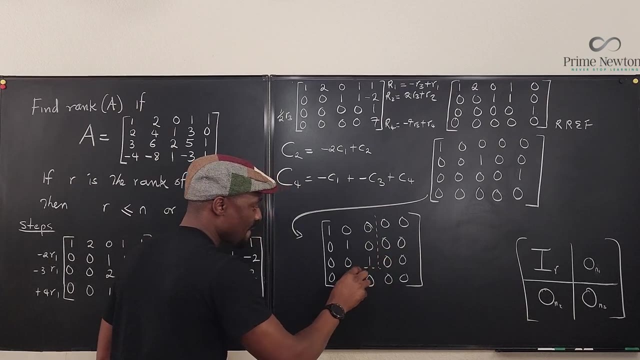 And then I have 0, 0, 0, 0.. I have 0, 0, 0, 0.. This is what I just explained here. That's what you get. So now, what you have here is the identity matrix for 3x3 matrix. 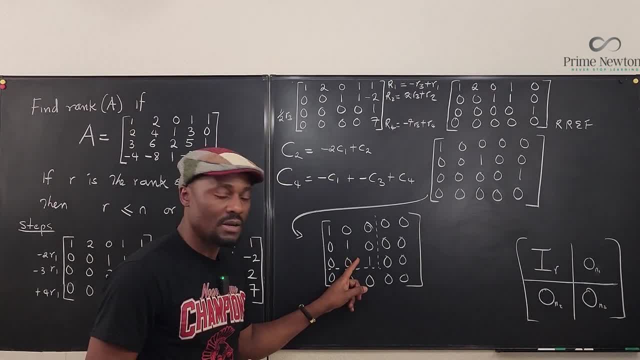 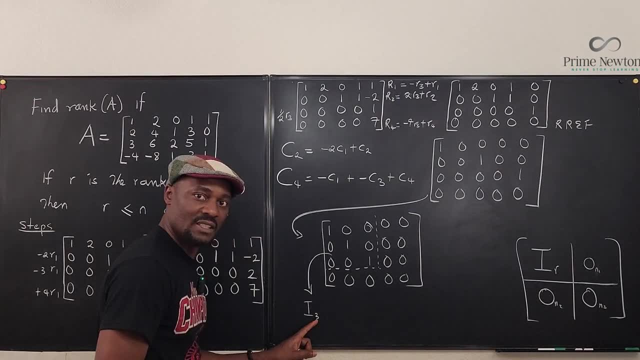 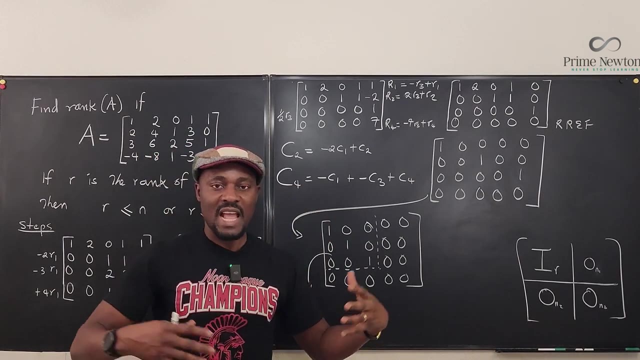 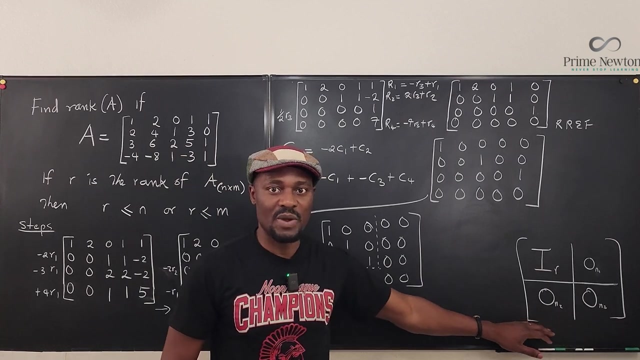 So this is I, sub R, This is I, This here is I sub 3, and your 3 is the rank of the entire matrix. So you want to practice and get good understanding of this whole idea. This is a theorem, by the way. 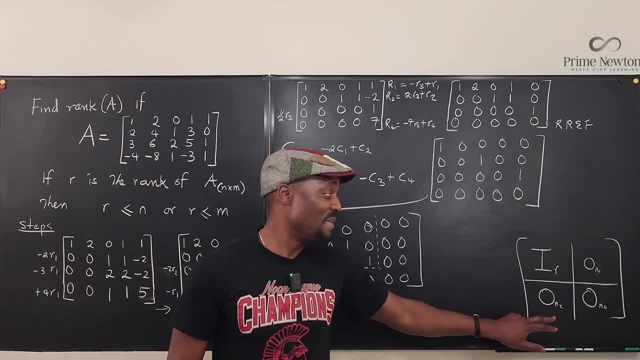 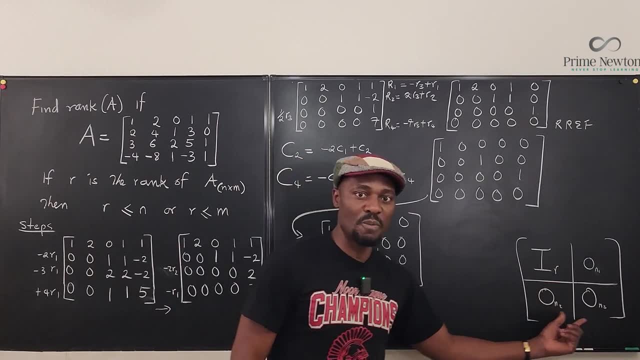 Actually, this is the theorem that I was talking about. This is the main theorem that all matrices can be written in this form, where R is the rank of the matrix, And these are all zero matrices of different dimensions, depending on how many zeros you have. 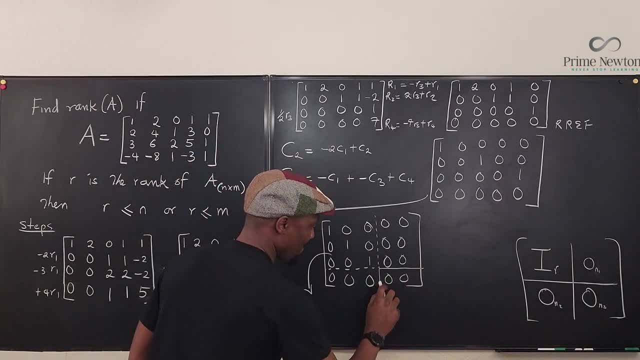 For example, if we classify this, this is what this is: This is a zero matrix. It is a 1x3 matrix. This is a zero matrix. It is a 1x2 matrix. This is a zero matrix. It's a 3x2 matrix. 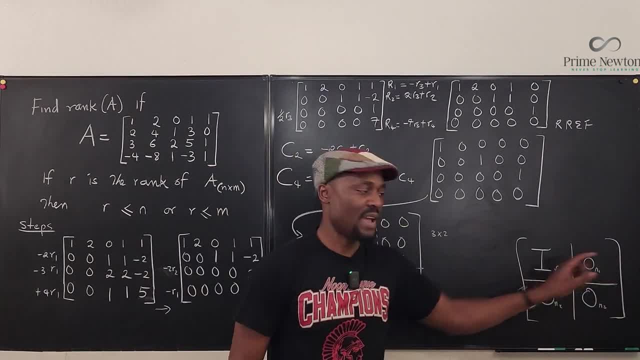 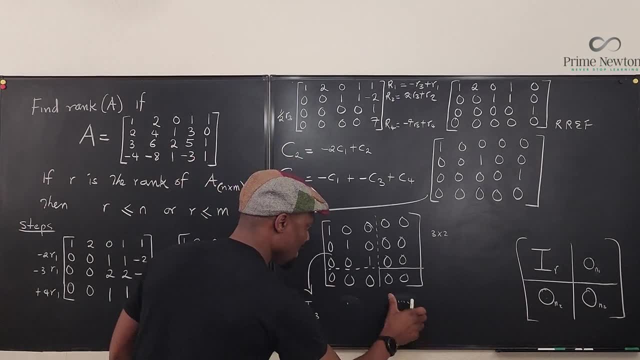 And that's what I had there. Maybe my notation is not perfect, but this one is what you need to know. OK, so the rank of the matrix? OK implies- let's get rid of this- This implies rank of A equals 3.. 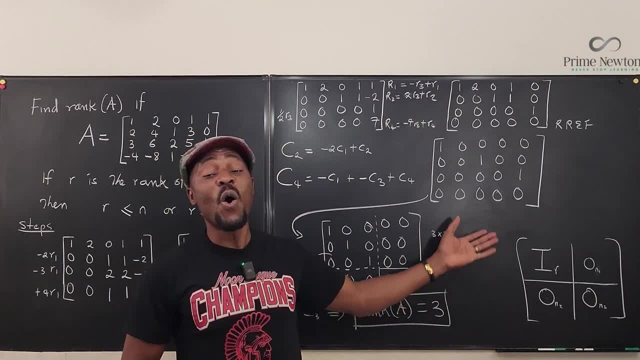 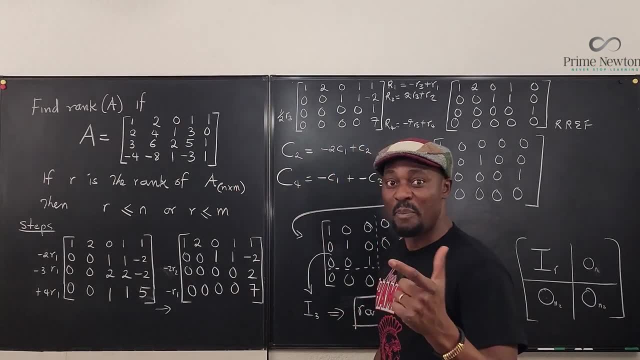 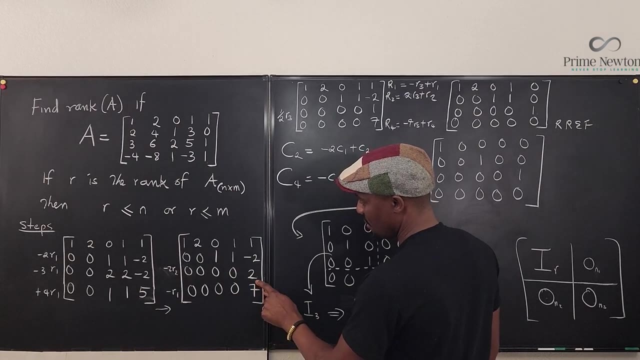 Remember, we didn't have to go all the way in order to discover what the rank is. In fact, as soon as you found out how many pivots there are. this is the first one, This is the second And this This is the third pivot. 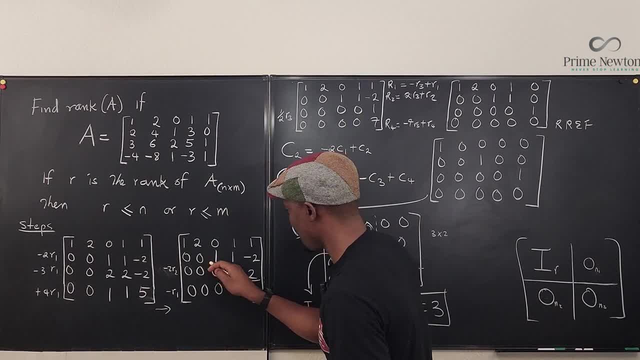 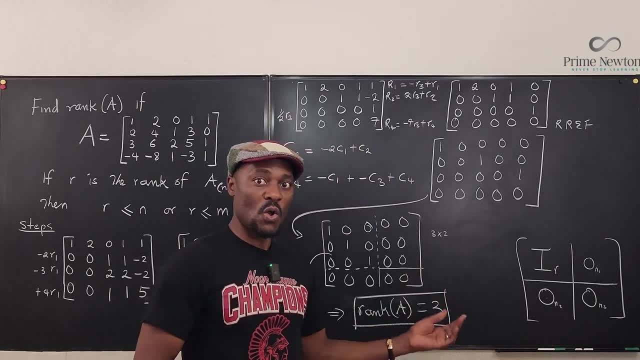 OK, these are your pivots. Once you find out your pivots, you know what the rank is. But if you need to show your work all the way, this is what you must do. Never stop learning. Doesn't stop learning stops living. Bye, bye.